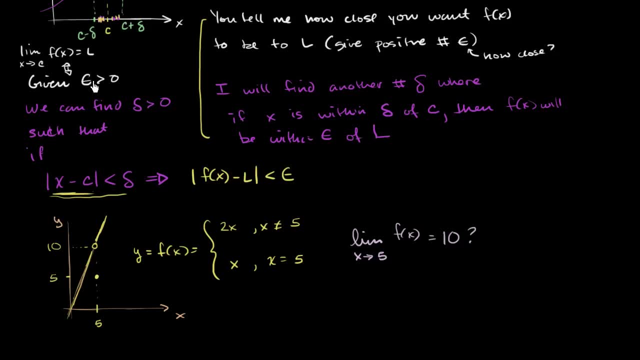 this essentially tells us how close we want f of x to be to l. we can always find a delta that's greater than 0.. It's essentially telling us our distance from c, such that if x is within delta of c, then f of x is going to be within epsilon of l. 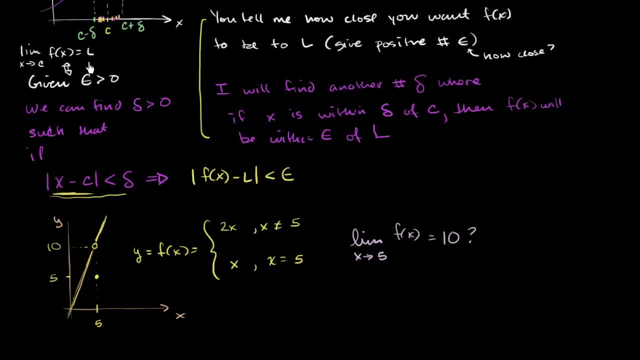 If we can find a delta for any epsilon, then we can say that this limit, that this is indeed the limit of f, of x, as x approaches c. Now I know what you're thinking. This seems all very abstract. I want to somehow use this thing. 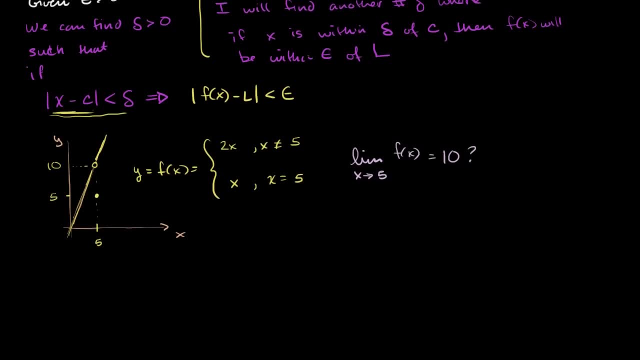 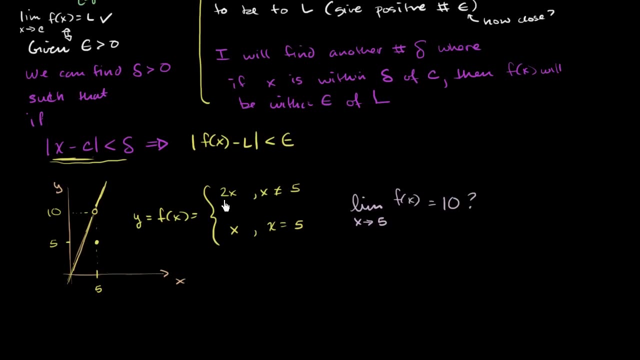 And what we will do in this video is use it and to rigorously prove that a limit actually exists. So right over here I've defined a function f of x. It's equal to 2x everywhere, except for x equals 5.. 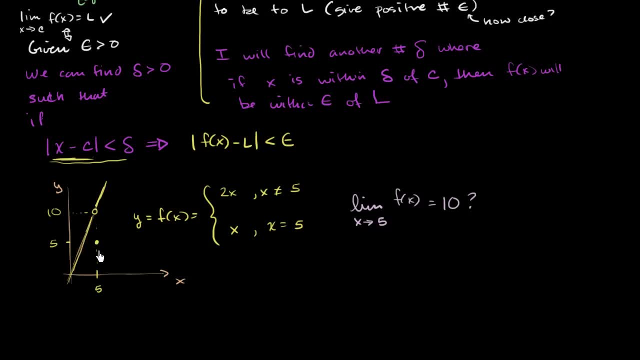 So it's 2x everywhere for all the other values of x. But when x is equal to 5, it's just equal to x. So I could have really just written 5 there. It's equal to 5 when x is equal to 5.. 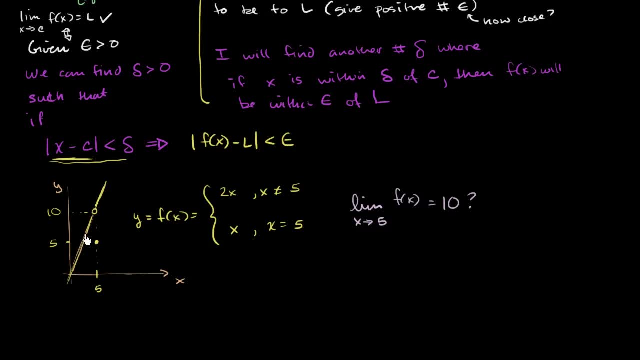 It's equal to itself, And so we've drawn the graph here. Everywhere else it looks just like 2x At x is equal to 5, it's not along the line 2x. Instead, the function is defined to be that function. 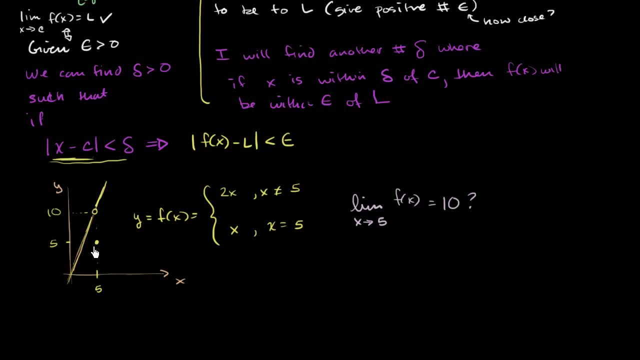 This point right over there. And if I were to ask you what is the limit of f, of x, as x approaches 5, you might think of it pretty intuitively. Well, let's see the closer I get to 5,. 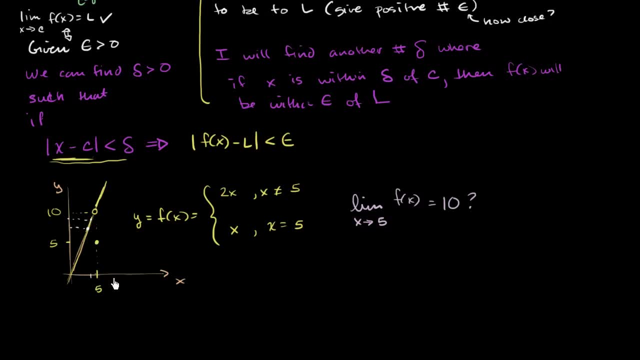 the closer f of x seems to be getting to 10.. The closer I get to 5,, the closer f of x seems to be getting to 10.. And so you might fairly intuitively make the claim that the limit of f of x as x approaches 5. 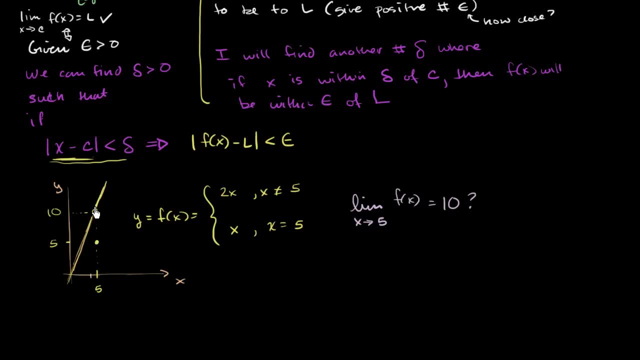 really is equal to 10.. It looks that way, But what we're going to do is use the epsilon-delta definition to actually prove it, And the way that most of these proofs typically go is we define delta in the abstract And then we essentially try to come up with a way. 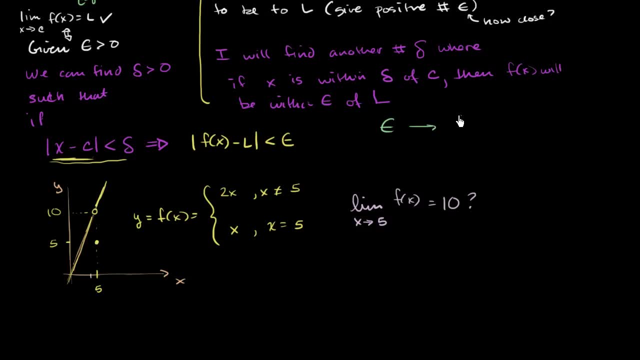 that, given any epsilon, we can always come up with a delta. Or another way is we're going to try to describe our delta as a function of epsilon- not to confuse you too much, But maybe I shouldn't use f again- But delta equals function of epsilon. 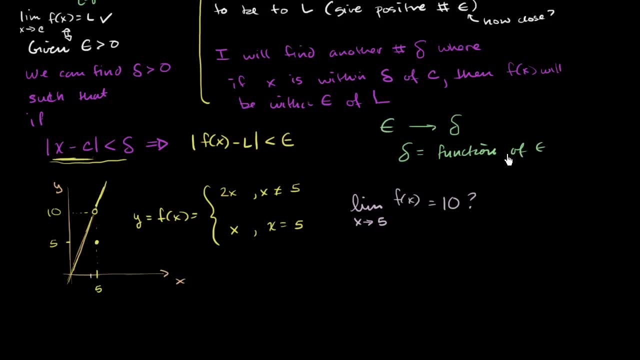 that is defined for any positive epsilon. So you give me an epsilon, I just put it into our little formula, our little function box, and I will always get you a delta. And if I can do that for any epsilon, that will always give you a delta. where this is true. 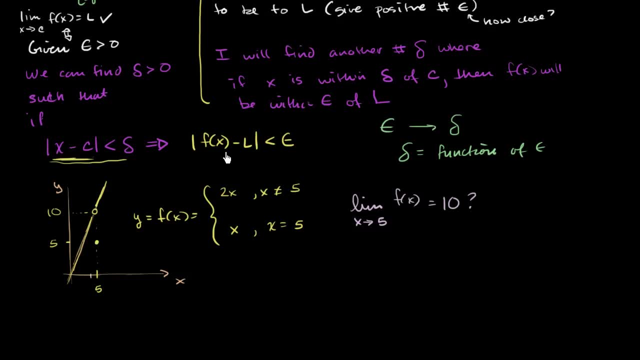 that if x is within delta of c, then the corresponding f of x is going to be within epsilon of l, then the limit definitely exists. So let's try to do that. So let's think about being within delta of our c. So let's think about this right over here as 5 plus delta. 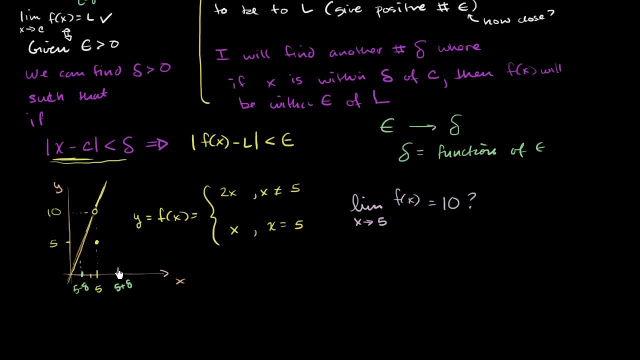 This is 5 minus delta. So that's our range we're going to think about, And we're going to think about it in the abstract at first, And then we're going to try to come up with a formula for delta in terms of epsilon. 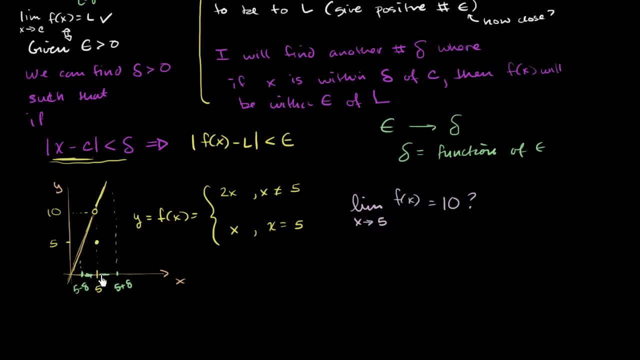 So how can we describe all of the x's that are in this range but not equal to 5 itself? Because we're really care about the things that are within delta of 5, but not necessarily equal to 5.. This is just a strictly less than. 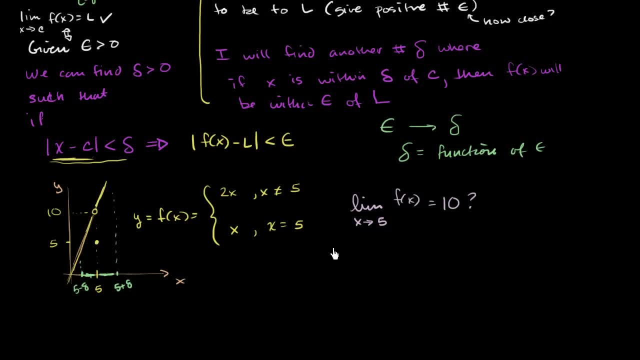 They're within a range of c but not equal to c. Well, that's going to be all of the x's that satisfy. x minus 5 is less than delta. That describes all of these x's right over here. Now, what we're going to do and the way these proofs typically. 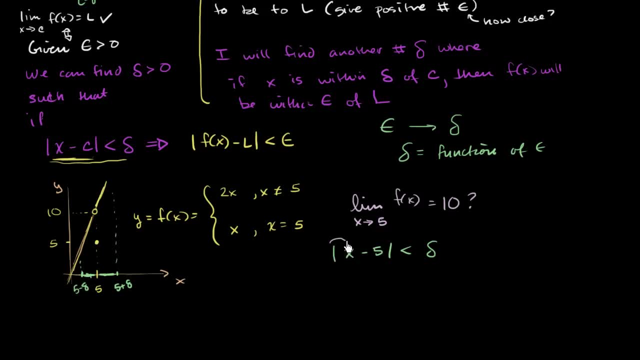 go is: we're going to try to manipulate the left-hand side of the inequality so it starts to look something like this, or it starts to look exactly like that, And as we do that, the right-hand side of the inequality is going to be expressed in terms of delta. 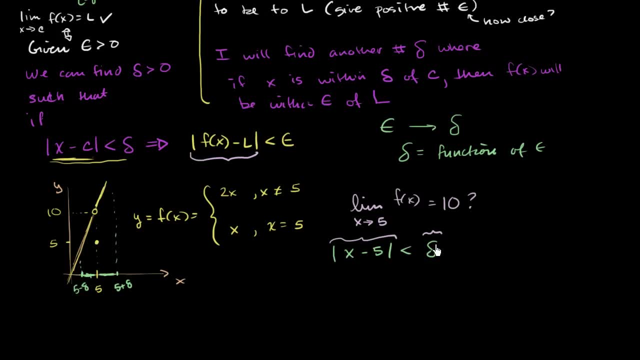 And then we can essentially say: well, look, if the right-hand side looks like delta or is in terms of delta, and the left-hand side looks just like that. that really defines how we can express delta in terms of epsilon. If that doesn't make sense, bear with me. 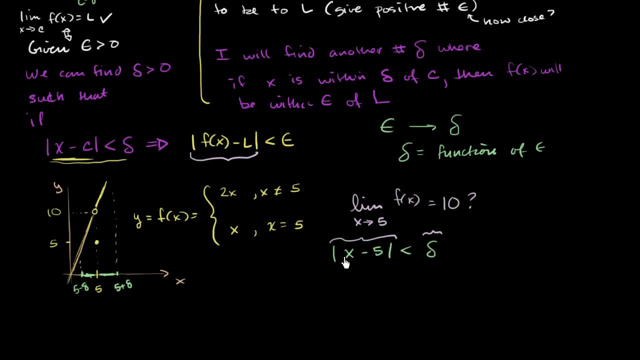 I'm about to do it. So if we want x minus 5 to look a lot more like this: when x is not equal to 5, and all of this whole interval, x is not equal to 5,, f of x is equal to 2x, our proposed limit is equal to 10.. 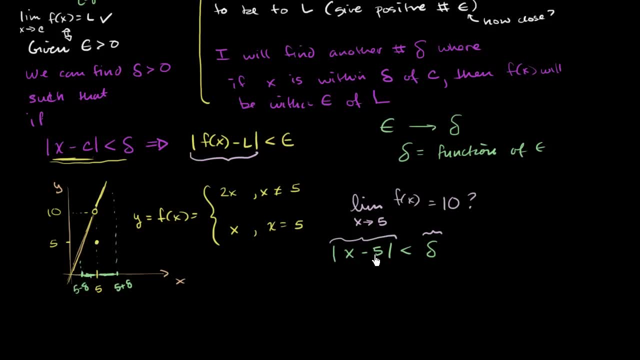 So if we could somehow get this to be 2x minus 10, then we're in good shape, And the easiest way to do that is to multiply both sides of this inequality by 2.. You multiply both sides of this inequality by 2.. 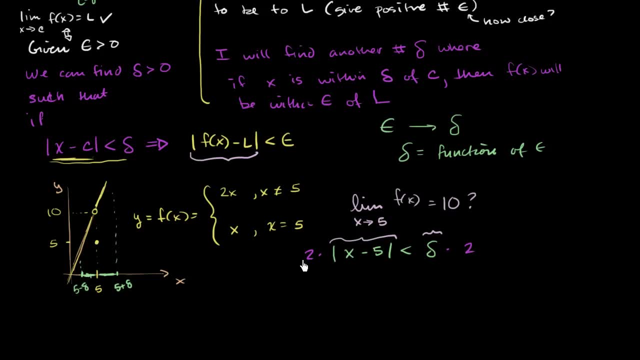 And 2 times the absolute value of something, that's the same thing as the absolute value of 2 times x. That's that thing. If I were to say 2 times the absolute value of a, that's the same thing as the absolute value of 2a. 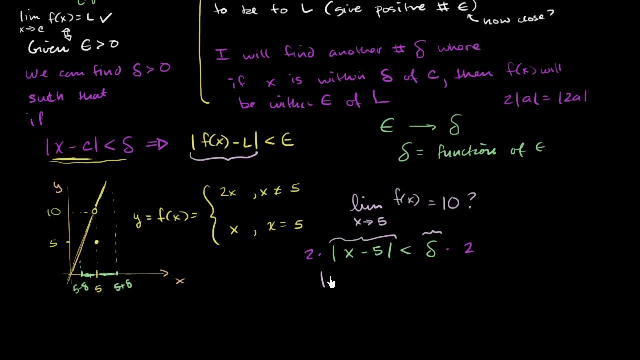 So on the left-hand side, right over here, this is just going to be the absolute value of 2x minus 10. And it's going to be less than on the right-hand side. You just end up with a 2 delta. 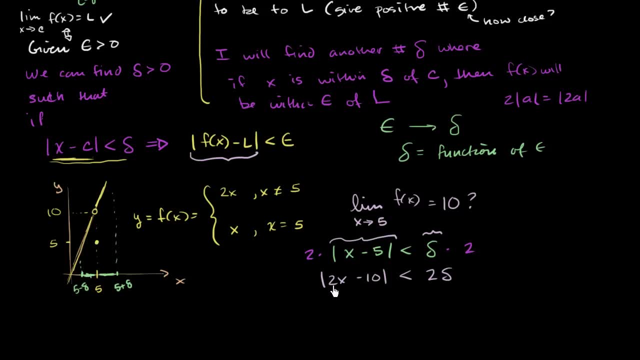 Now, what do we have here on the left-hand side? Well, this is f of x, as long as x does not equal 5.. And this is our limit, So we can rewrite this as f of x minus l. This is less than 2 delta. 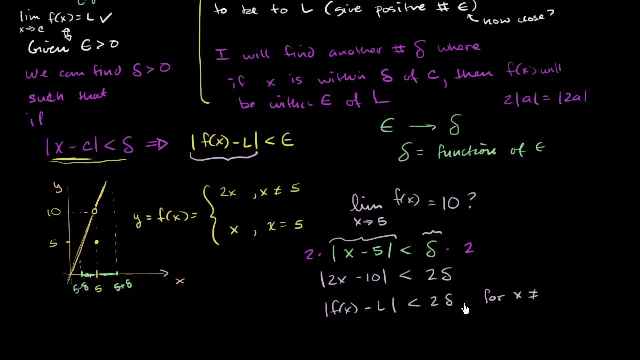 And this is for x- does not equal 5.. This is f of x. This, literally, is our limit. Now this is interesting. This statement right over here is almost exactly what we want right over here, except the right sides are just different. 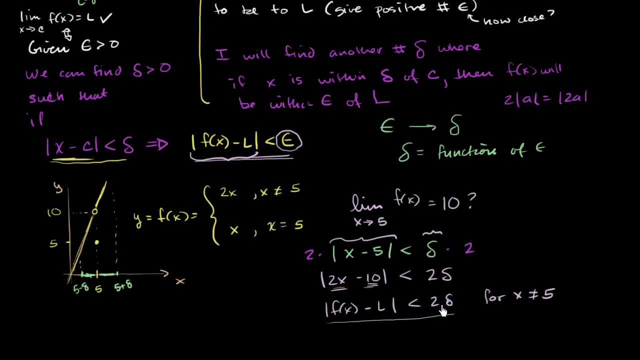 This has in terms of epsilon, this has it in terms of delta. So how can we define delta so that 2 delta is essentially going to be epsilon? Well, this is our chance. We will just define, And this is where we're defining delta as a function of epsilon. 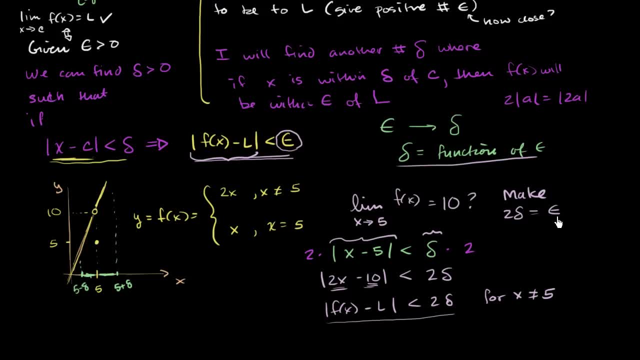 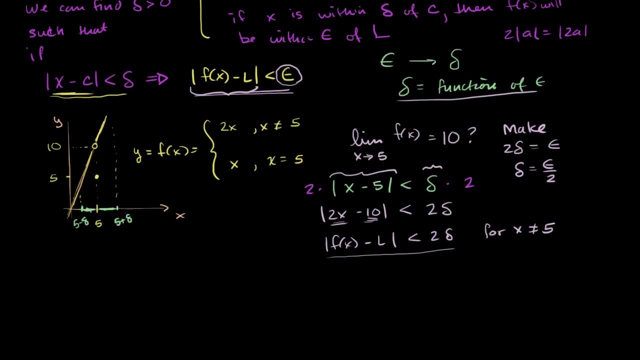 We're going to make 2 delta equal epsilon. Or if you divide both sides by 2, we're going to make delta equal to epsilon over 2.. So if you make delta equal epsilon over 2, let me switch colors just to ease the monotony. 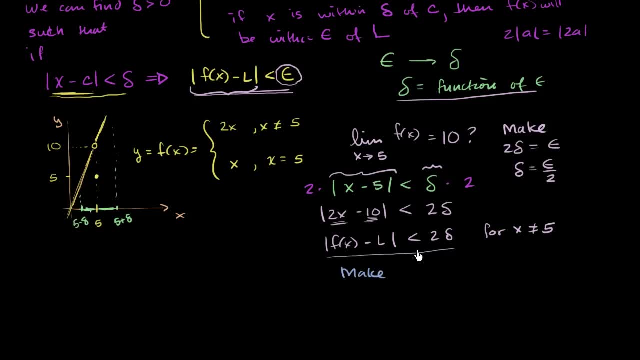 Let me switch colors just to ease the monotony. If you make delta equal epsilon over 2, then this statement right over here becomes: the absolute value of f of x minus l is less than. Instead of 2 delta, it'll be less than.